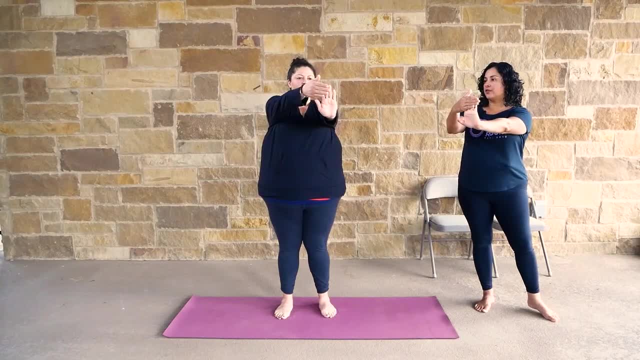 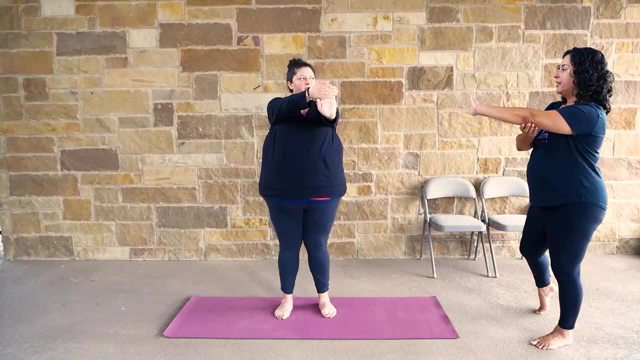 fingers up and take a hold of your- just right across all of your fingers- and draw them back gently. So here you may be, feeling stretching happening in your fingers, your palm and the underside of your arm, And we'll just stay here for a 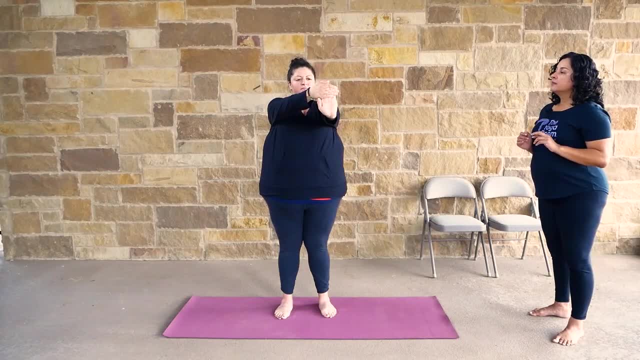 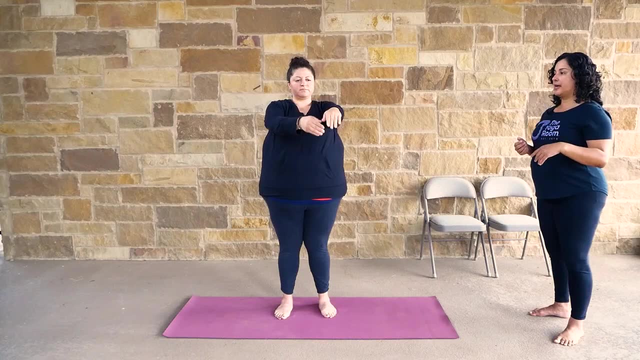 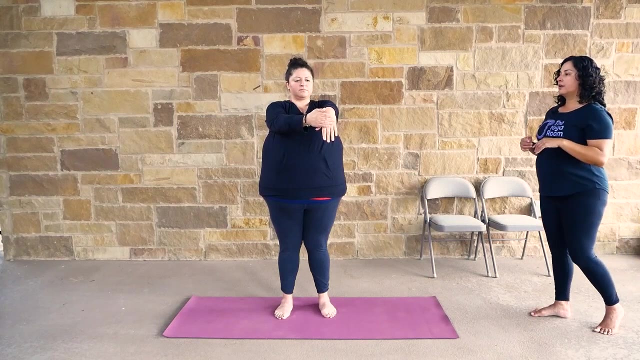 few breaths. Okay, when you're ready, you can release that, point your fingers down and now take a hold of the back of your hand rather than your fingers, And we're going to do the same. just a little bit of pressure, There you go, And now you may be feeling. 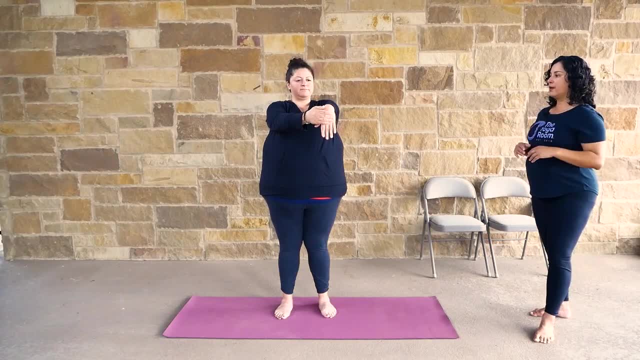 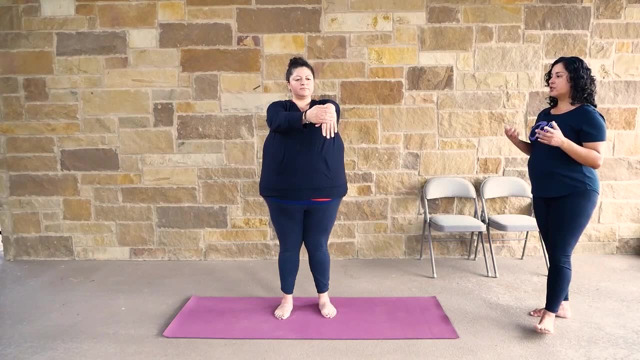 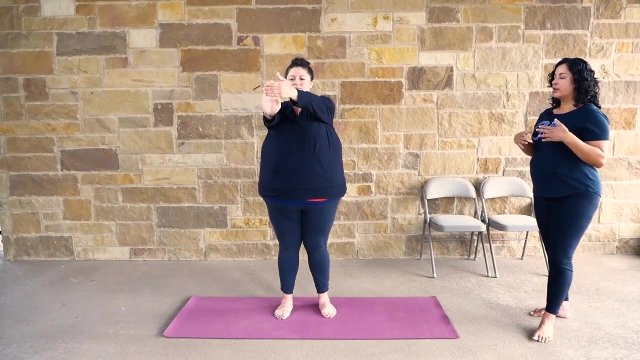 stretching happening in the back of your hand and the top side of the forearm. Okay, let's go ahead and switch to the other side. So now, right fingers point up and down, Take a hold of them, draw them back, And so, in the yoga practice generally, we're 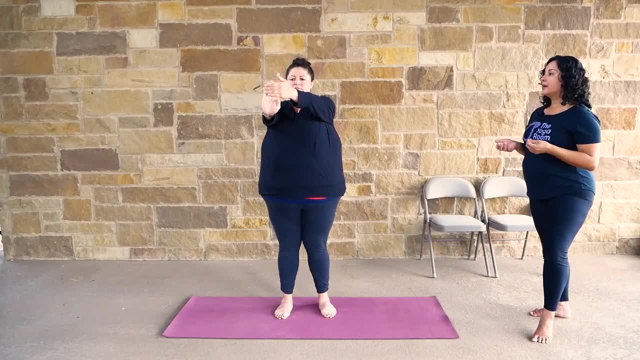 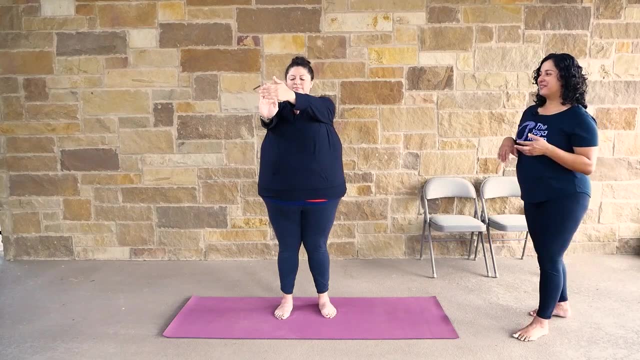 trying to inhale and exhale smoothly in and out through the nose if it's comfortable. If you need to, you can breathe through your mouth. if you're congested on any given day, Okay, go ahead and release this one. Fingers point down. 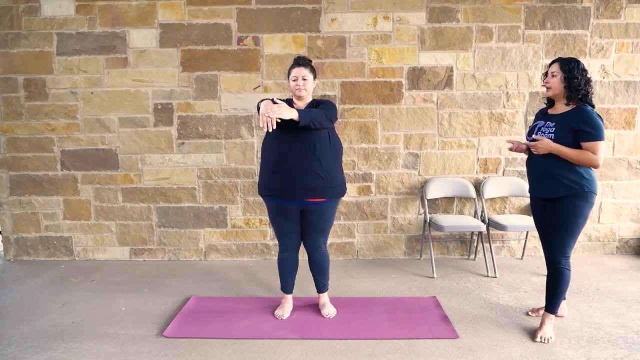 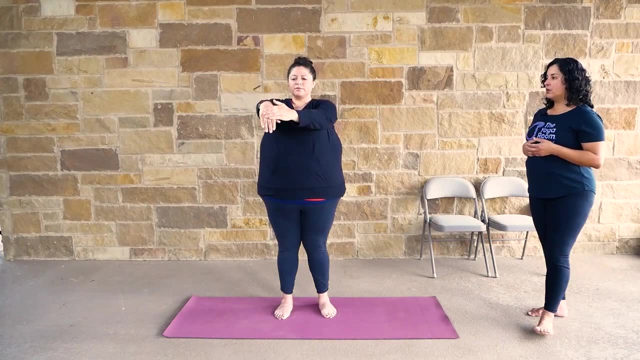 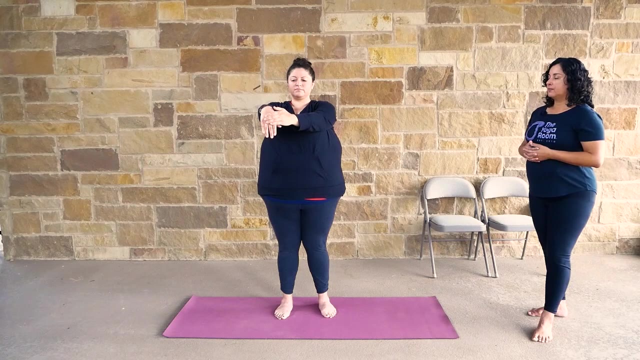 take a hold of the back of your hand and let's spend about three breaths here, Just like I described: smoothly inhaling through the nose, exhaling through the nose and then out. Continue relaxing your shoulders down And, after those three breaths are done, you can relax your arms down, shake your 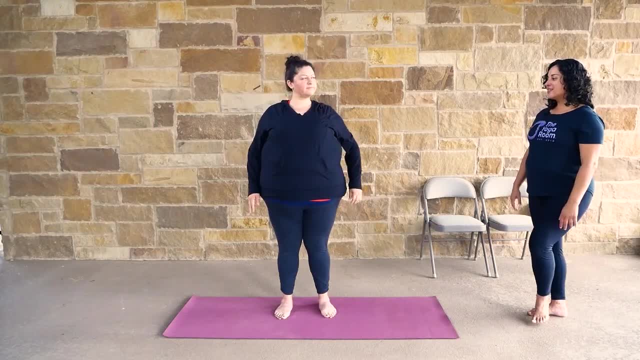 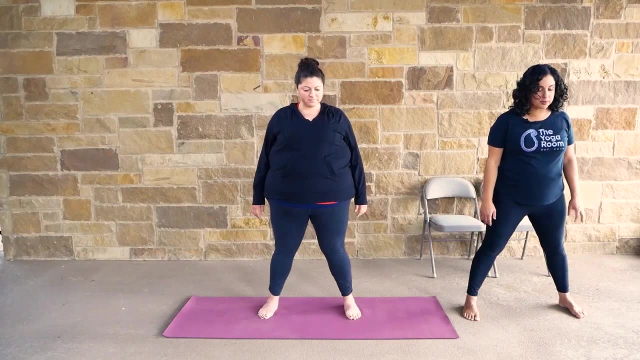 hands out a little bit. Very good work. Next, let's start to work on some side bending to stretch out the sides of the body. So step your feet wide, any width that's comfortable for you, Lengthen your spine again and then stretch out the. 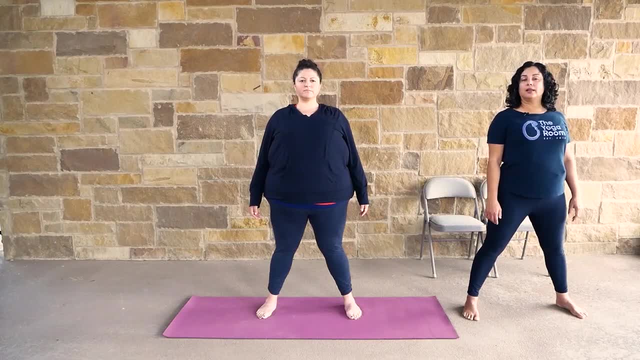 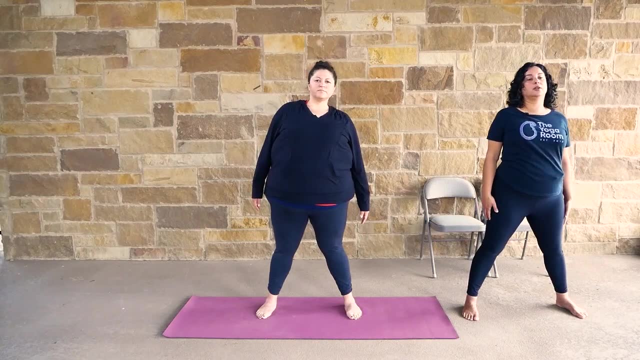 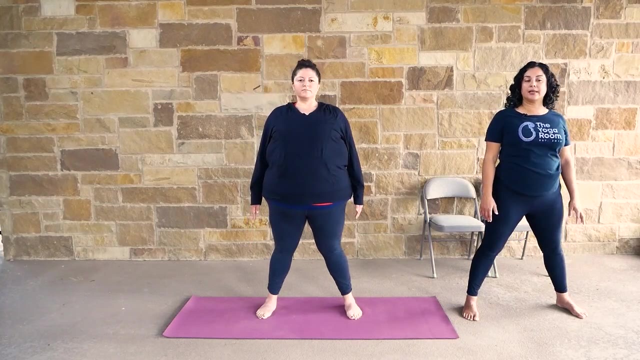 shoulders. Again, relax your shoulders, Then inhale. lengthen your spine tall. Exhale side: bend toward the left. That's it. Inhale to the center. Exhale side bend toward the right. Inhale to the center And then exhale and relax And we're gonna. 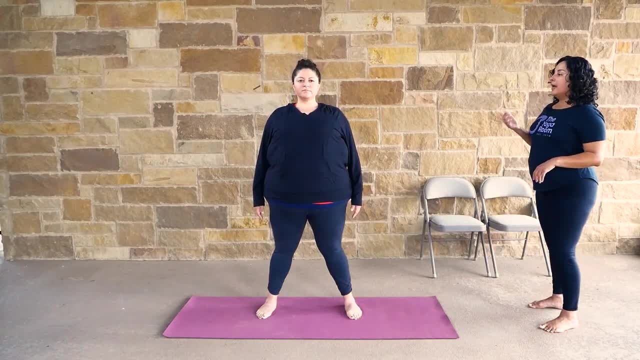 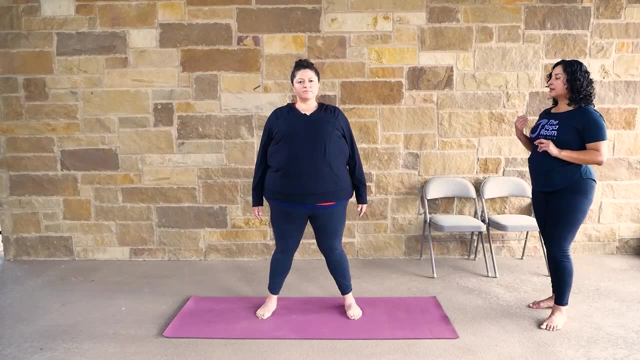 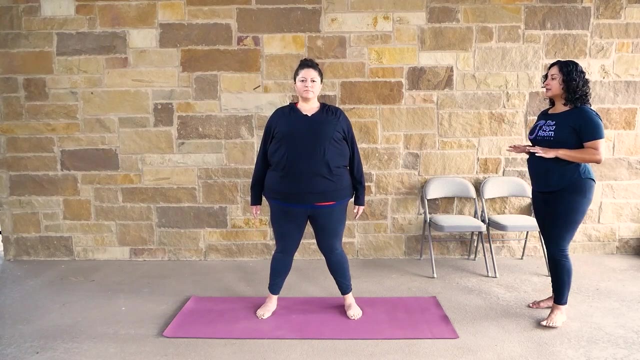 to do it again. Inhale, lengthen your spine. Exhale side bend left. Inhale to the center. Exhale side bend right. Inhale to the center. Exhale- relax. Go ahead and keep going. Do two. 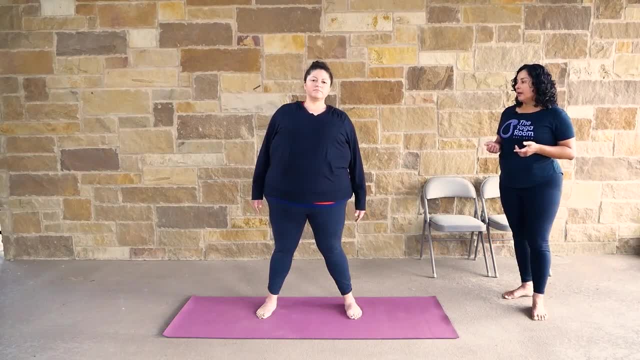 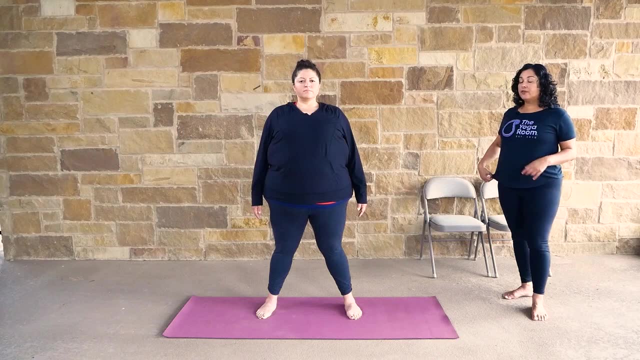 more, Go at your breathing pace And some other things that you may be feeling when you do this movement. you know primarily we're stretching out in the sides of the body, But if you're a person who has tightness in your back, you may also be feeling a little bit of relief happening. 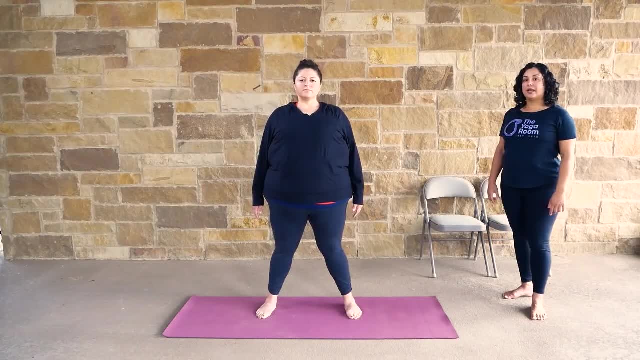 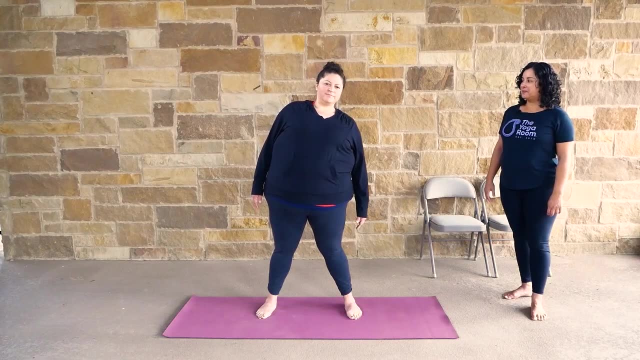 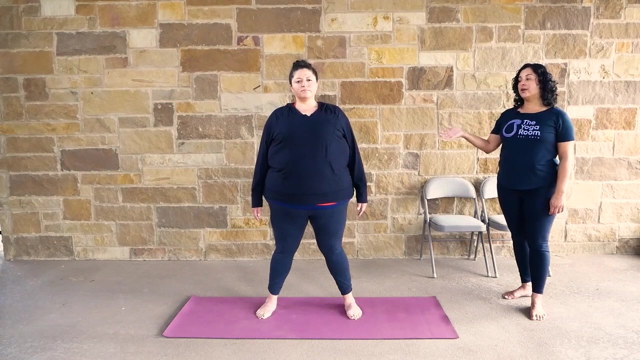 in your low back, the back of your hips, sometimes even in the upper back and shoulders. We're going to do one more, All right. One thing Denise is doing really well here is she's bending to the side only, without forward bending. Sometimes that happens. 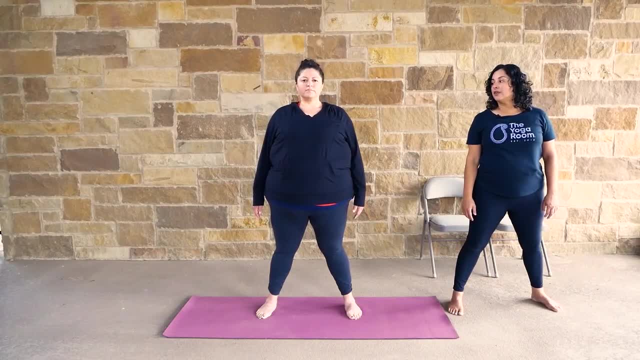 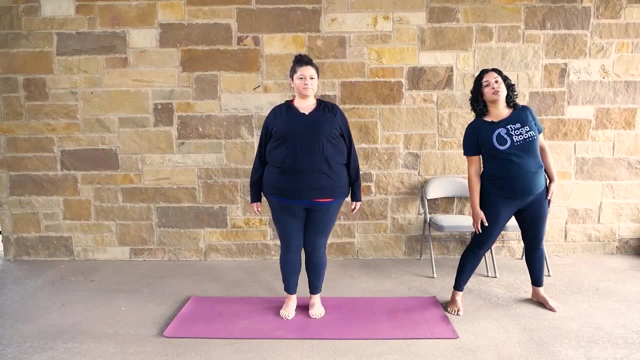 Especially if we're feeling tight. Whenever you finish, just rest here. You can step your feet together if you want to. But what I was saying is sometimes, if our body feels really tight and we try to side bend, we end up also forward folding. So go to the range, that's. 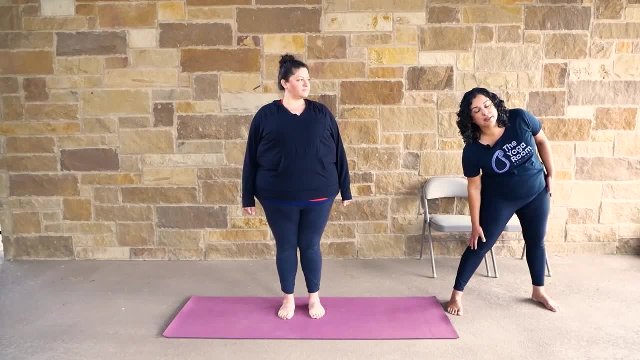 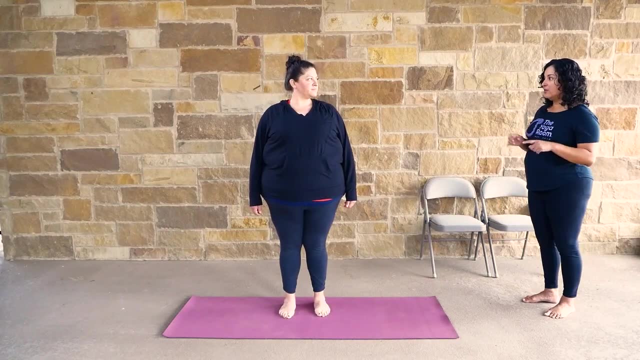 comfortable for your body and just be mindful that you're not also inadvertently folding forward. All right, Feeling okay. All right, Let's continue. So the next thing we're going to work on is forward folding, And I know that you are very flexible, but not everybody is, So we're 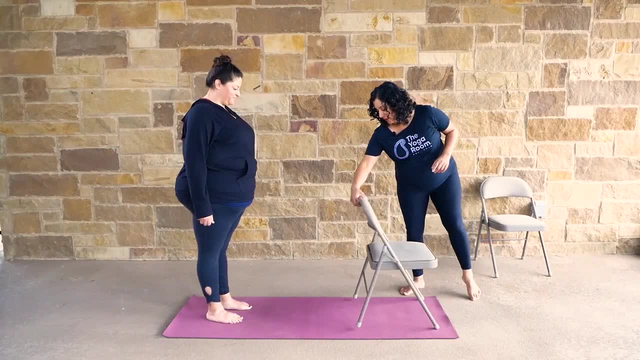 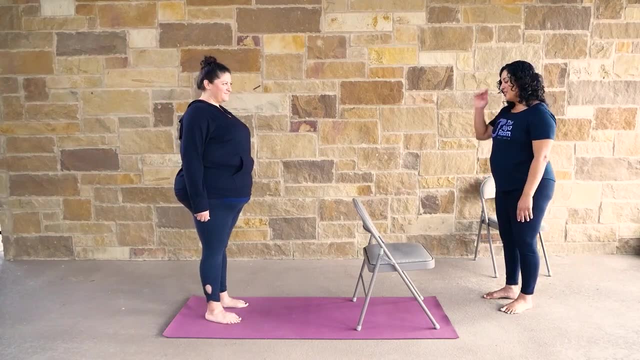 going to try a modification for forward folding today And we're going to use a chair, And if you find you don't need the chair, you absolutely don't have to use it. You can bring your hands onto your legs instead. So step forward just a little bit. There you go. I think that should be. 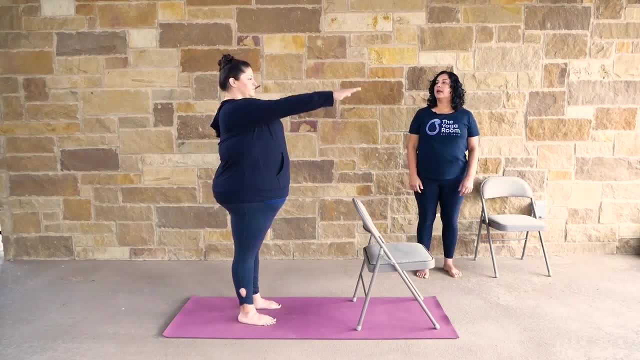 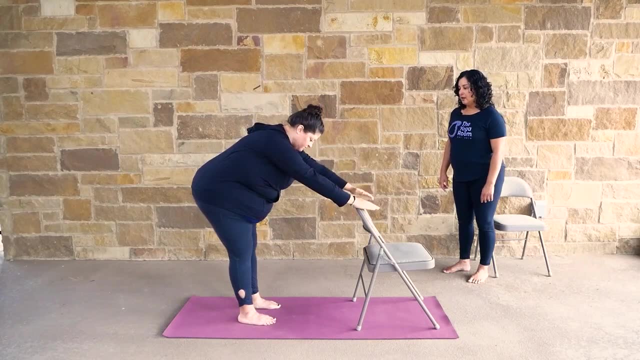 okay, Inhale. Bring your arms forward and up. Palms will face front. Exhale. Bend your knees and you can bring your hands to rest on the back of the chair. Fold as much as you're comfortable. Relax your neck. Wonderful, Then inhale. 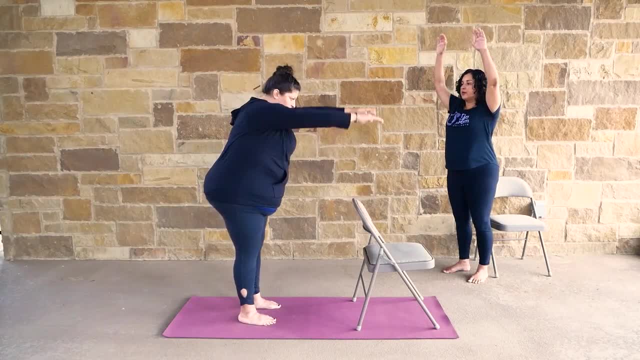 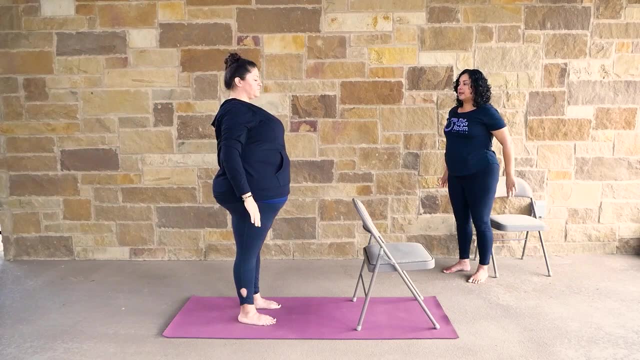 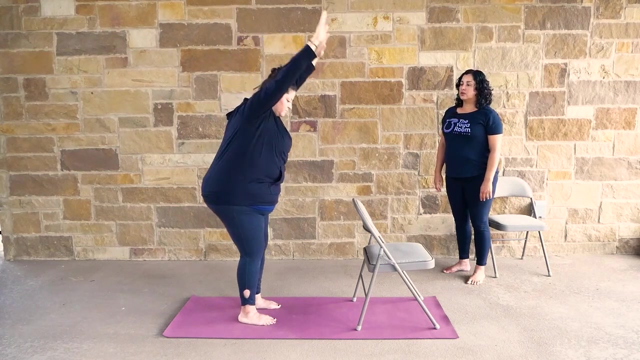 Come up again. If it's comfortable for you, you can raise your arms overhead And then exhale. Just your arms move forward and down. Let's do another one like this: Inhale Arms forward and up, Exhale and fold to your comfort level. 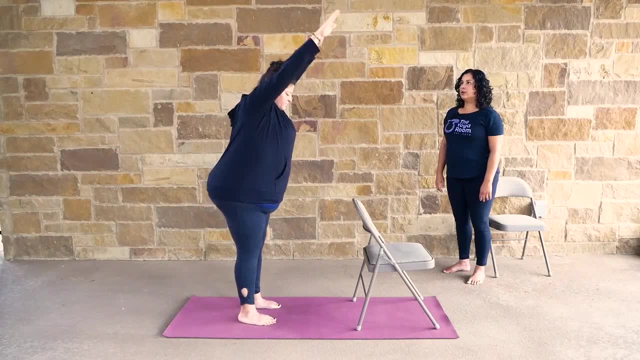 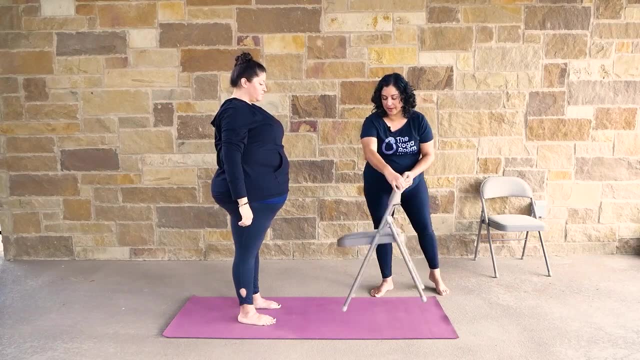 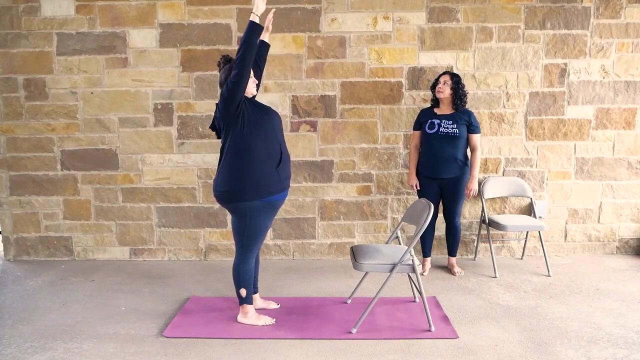 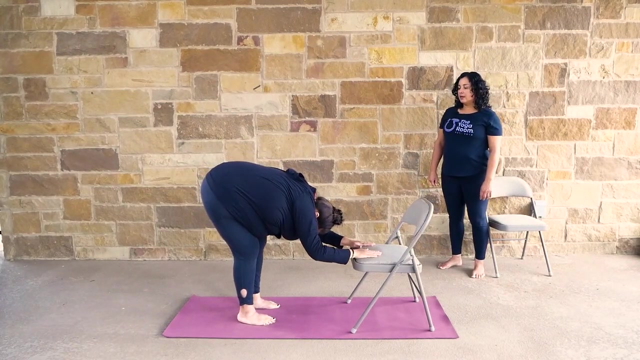 Inhale Come up. Arms can reach overhead if it's comfortable. Exhale Arms move forward and down. Okay, let's do another pair with a different modification. So now hands can go onto the seat of the chair if it's comfortable. Inhale Arms forward and up. Exhale Fold. Inhale Come up. 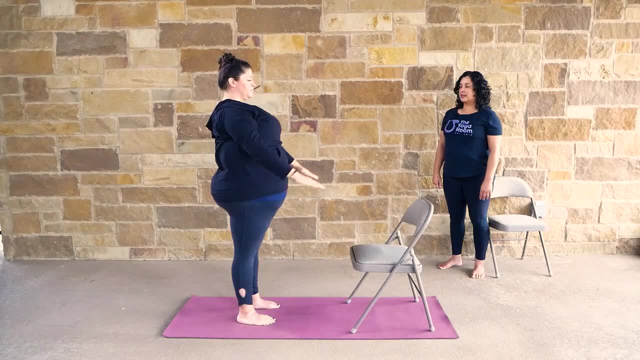 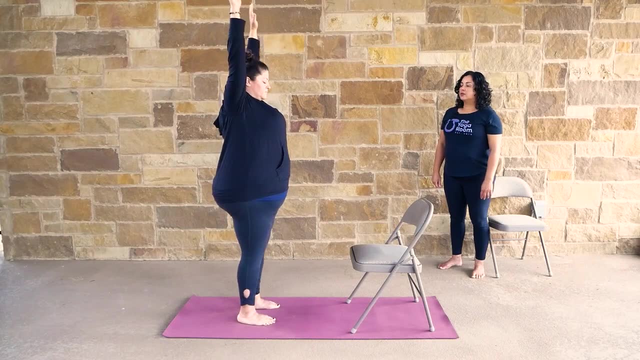 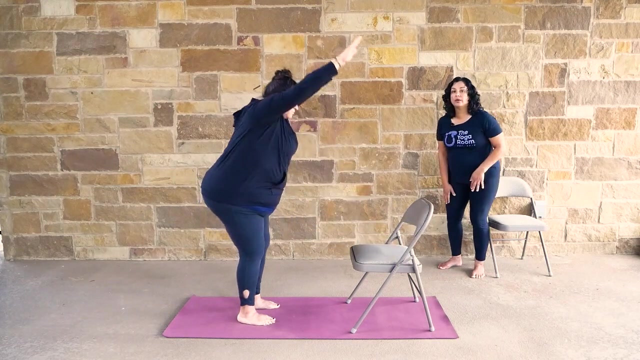 Exhale Arms forward and down. One more like this: Inhale Forward and up. Exhale, Fold, Inhale, Come up. You can either stretch your arms overhead or you can walk your hands up your legs. 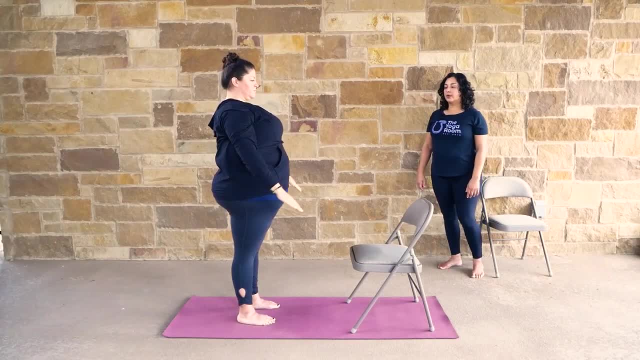 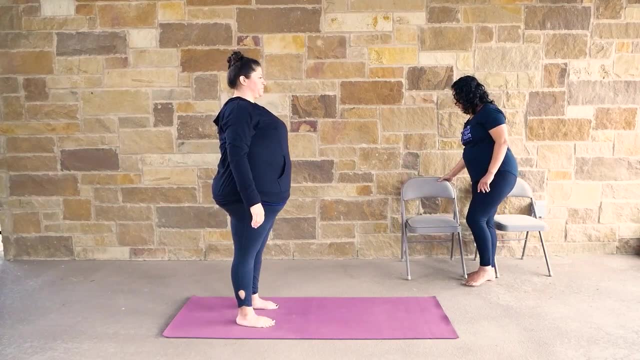 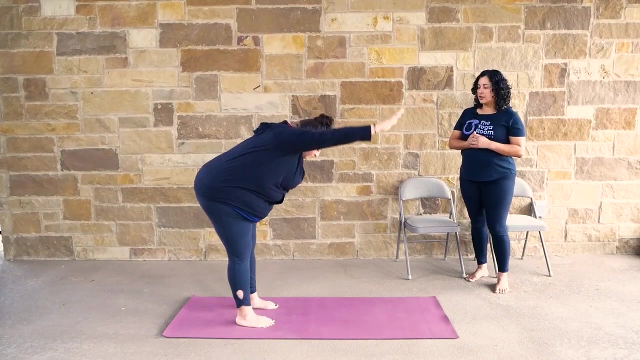 That's also fine. Exhale Arms forward and down. And if you're feeling really flexible today, you don't need a prop. We'll do two rounds of that variation as well. So that's: inhale arms forward and up. Exhale- Fold as much as you're comfortable. Hands can rest on your legs on the floor, Relax. 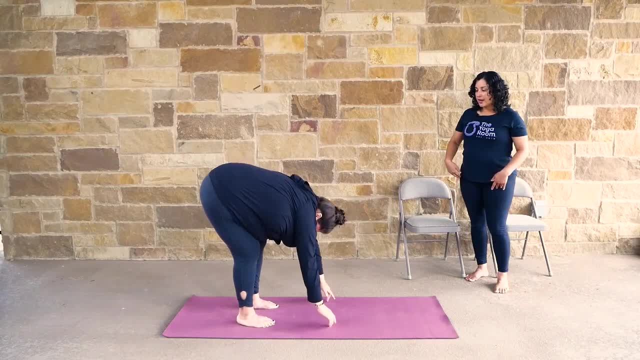 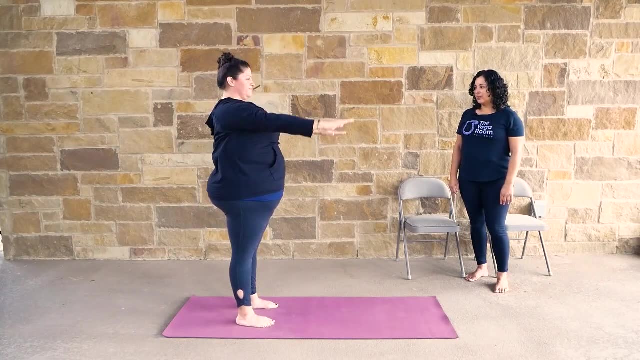 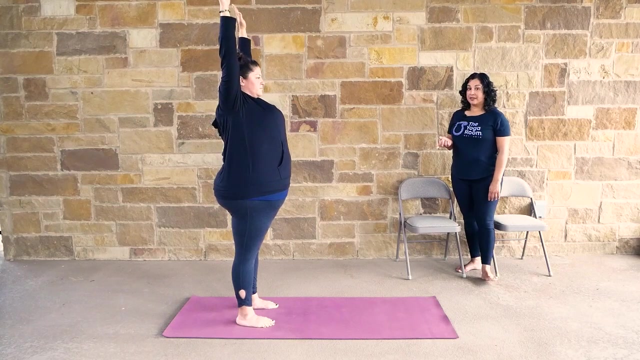 relax your neck, then inhale. come up, either walking your hands up your legs or stretching your arms forward and up. exhale arms forward and down. go ahead and do one more. go at your, your pace. so denise is not only flexible, but also very strong. if you aren't as strong as denise's yet, you may not be able to come up with your. 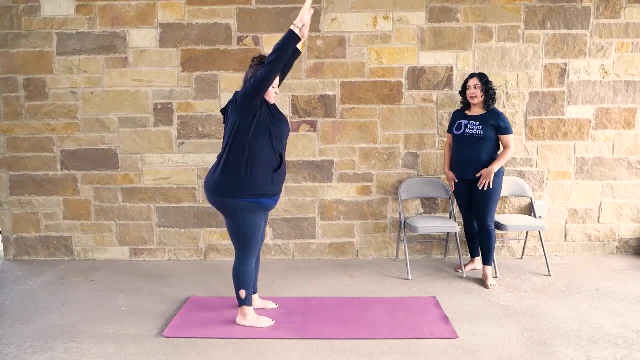 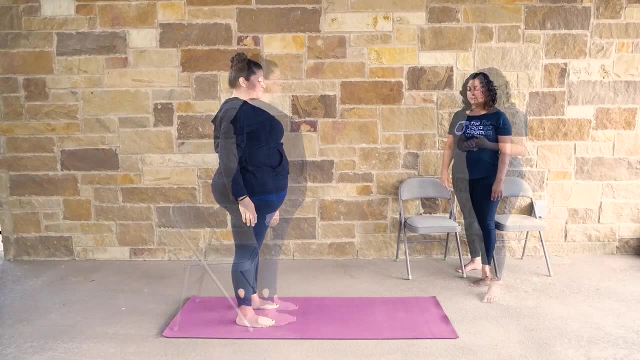 arms extended like she's doing, so please feel free to walk your hands up so that your back will be comfortable. very good work. okay, take a rest for just a minute here. next we're going to work on stretching out the backs of the legs using two chairs, so go ahead, please. and 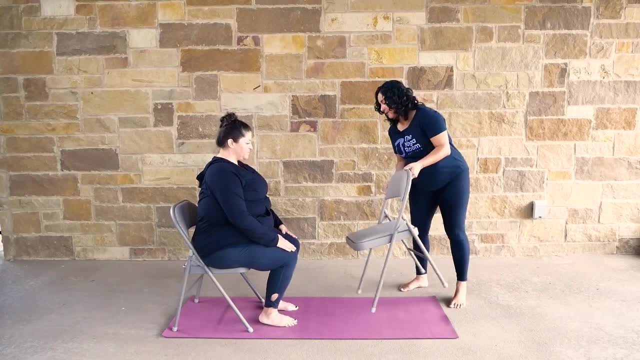 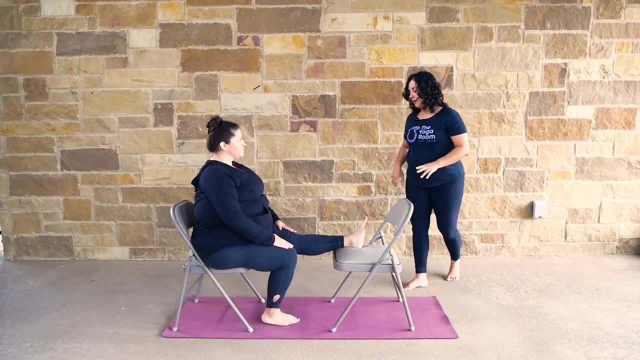 have a seat and i'm going to bring this chair right in front of you and you can bring your left leg up onto the chair. okay, that's great. i'm going to just pause here and explain for a minute, so this posture can be done sitting on a. 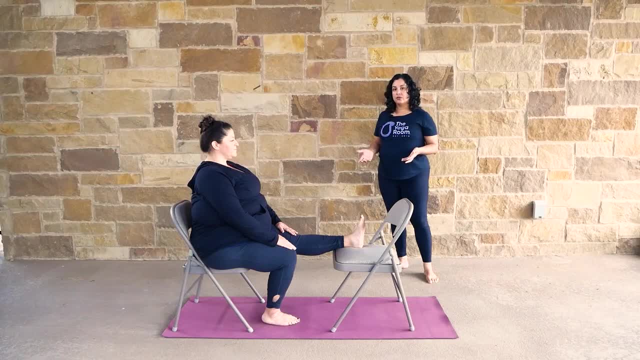 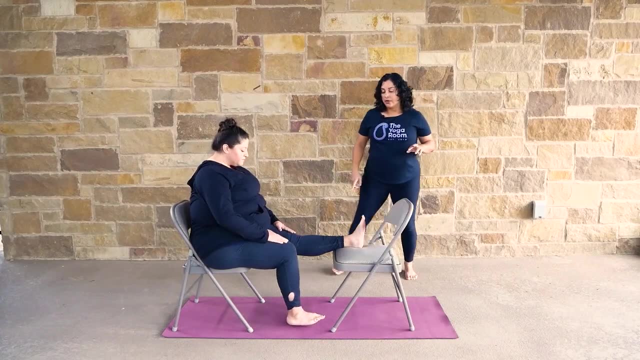 chair or, if you're comfortable getting down onto the floor, you can also do this sitting on the floor. the difference would be that, instead of having the right leg bent and the foot on the floor, you're going to have your right leg in about this position, something like this, when you're sitting. okay, so for this. 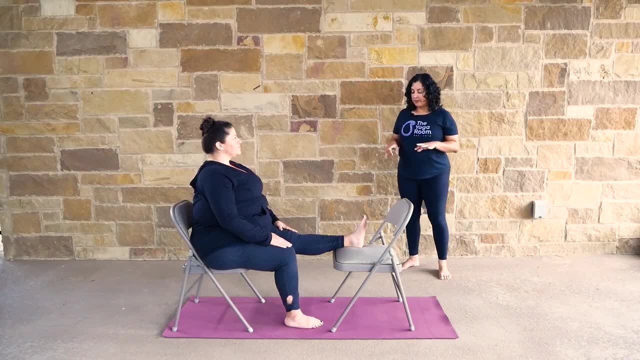 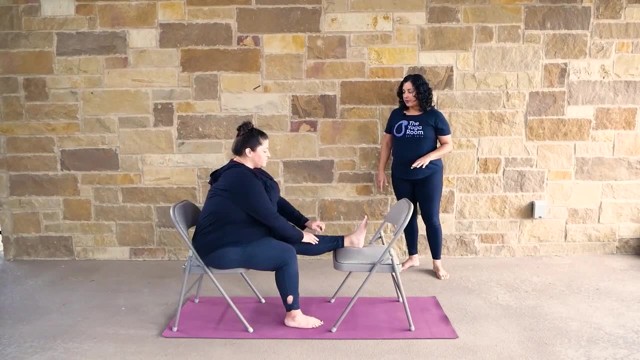 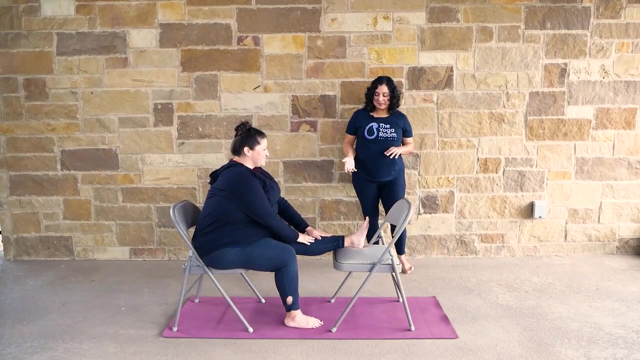 variation. are you comfortable here? okay, so we're going to work on some forward folding. let's do it in a static way, so just go ahead and walk your hands down your extended leg to your comfort level, and here you may feel a little bit more comfortable, a little or a lot of stretching in the back of your leg. 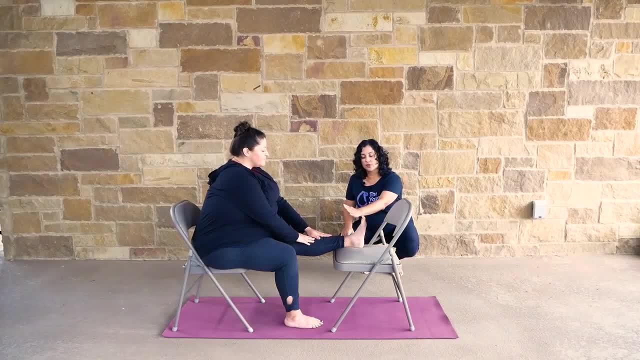 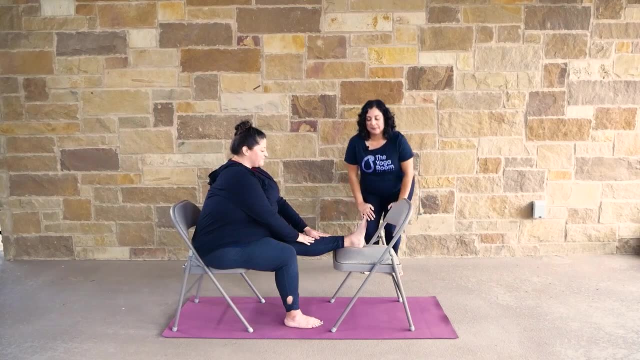 and you'll find that if you flex this foot, so in other words if you draw the toes back, this will increase the intensity a lot, so you can adjust the foot position accordingly. okay, when you're ready, go ahead and walk your hands up. take a break from this. 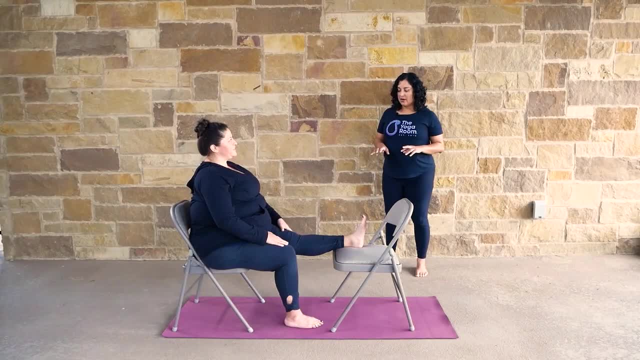 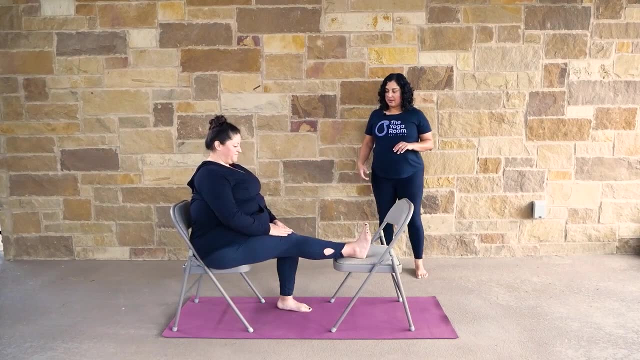 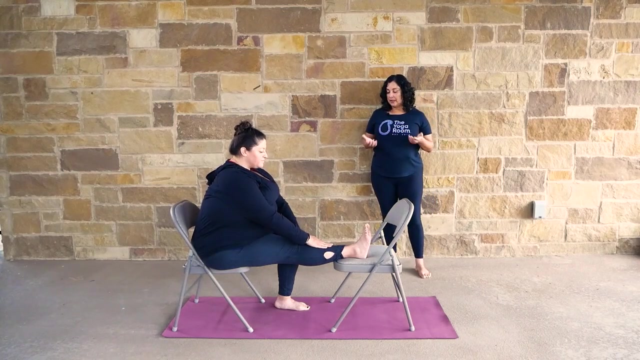 was it strong or is it okay? okay, all right, let's give it a break and let's work on the other side. so bring your right foot up and we'll do the same thing here: a little bit of forward fold. you might find that the two sides of the body feel completely different. 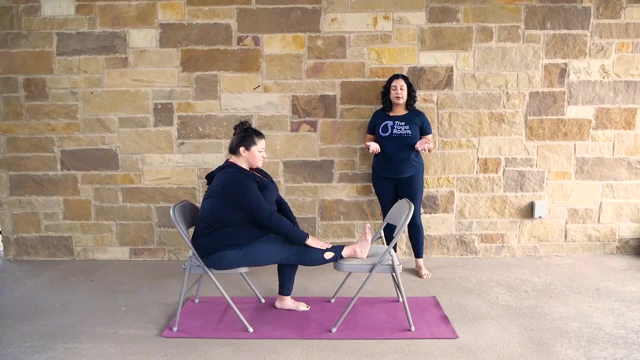 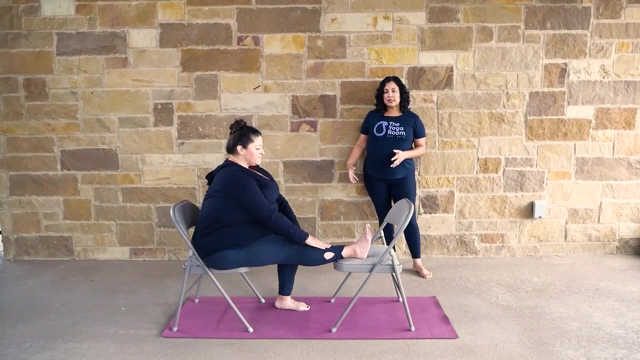 it really depends a lot on how you use your body throughout the day. so in the moment i realize that i'm standing leaning on this leg, if i have a habit of, you know, always leaning to the one side, there's a pretty good likelihood that this leg is going to feel tighter. 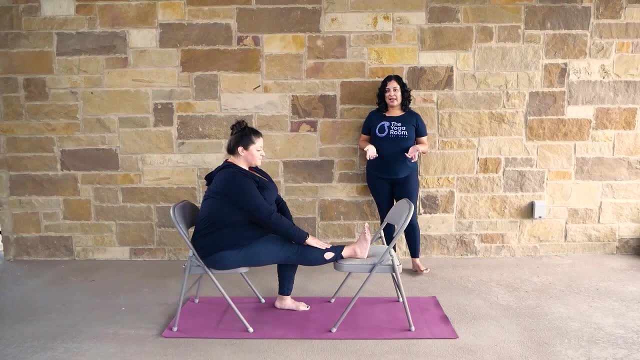 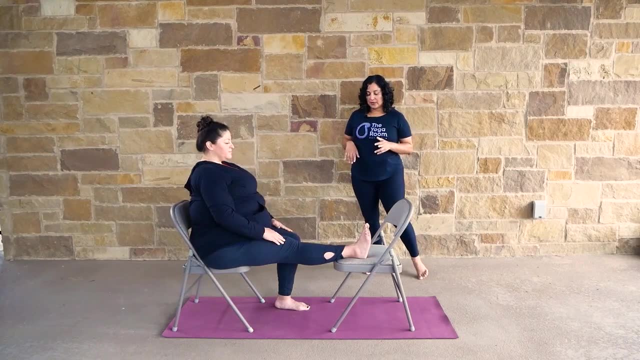 and you can notice that that kind of thing in your own daily habits and in how you're feeling when you do your yoga practice. okay, go ahead and come up, take a break from this one, set your foot down, and then we'll do one more round. so 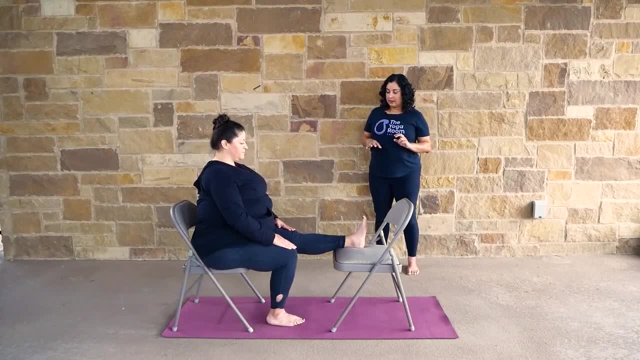 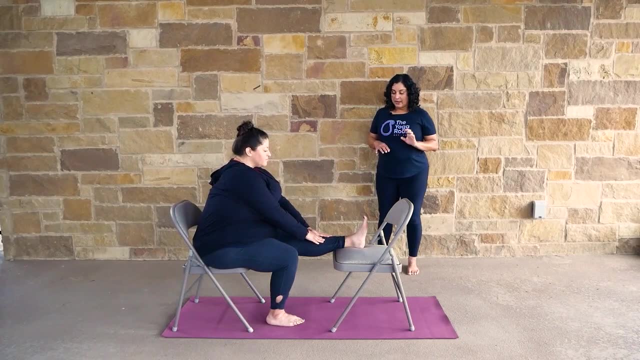 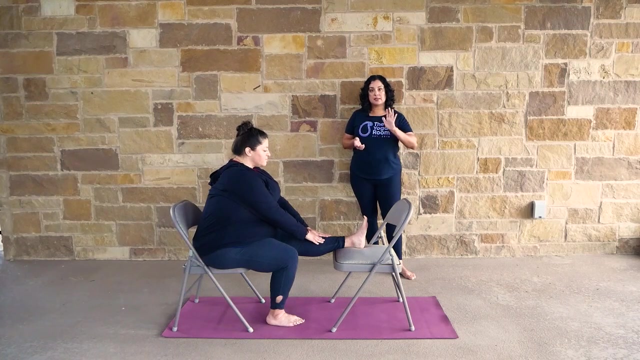 bring your left leg up again and again. a little bit of forward fold and the foot flexing, you know. kind of take it at your own pace. when you feel ready for a little more intensity, you can add that foot flex. if it's too intense, then just keep the foot relaxed. 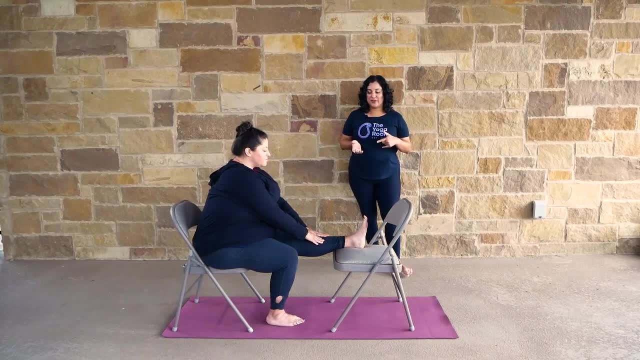 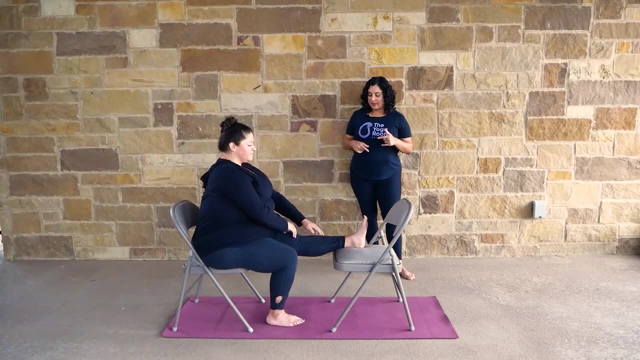 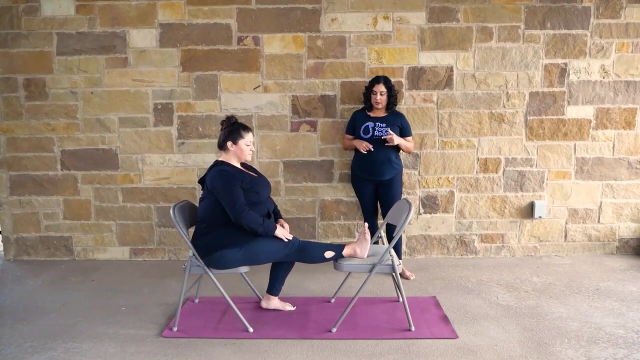 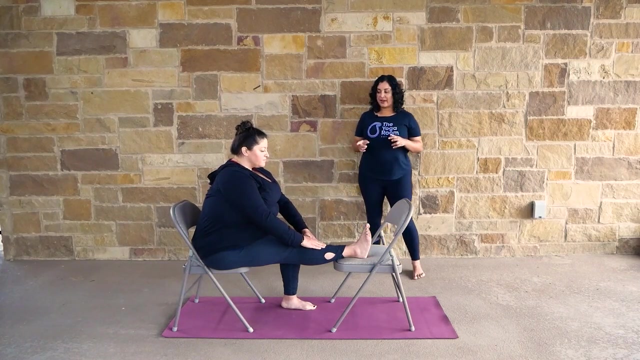 just remember that all of the yoga practice should feel comfortable. nothing should hurt, so you can adjust the practice accordingly. okay, when you're ready, go ahead and come up, set your foot down. we'll do one more round on the right side, okay, good, do you find one tighter than the other? they're equal. 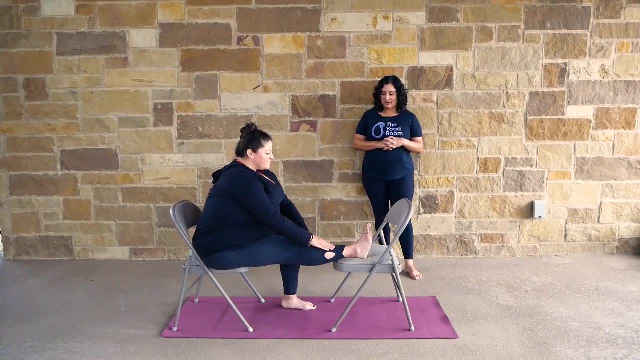 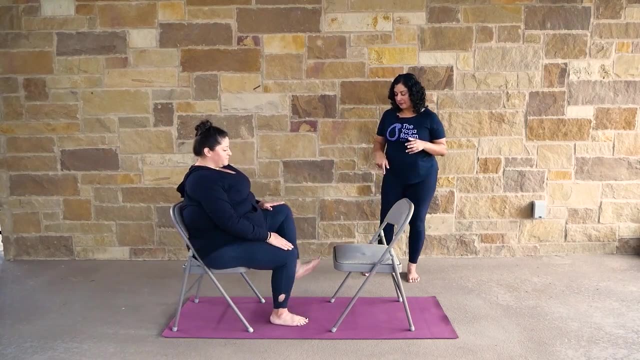 okay, wonderful, go ahead and come on up, and then let's show a second variation. so bring this foot down, bring your left foot up, and then what we're going to do is walk this right foot out toward the side a little bit. it might even come off your. 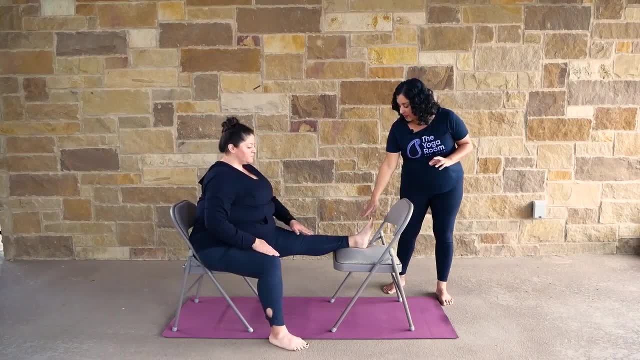 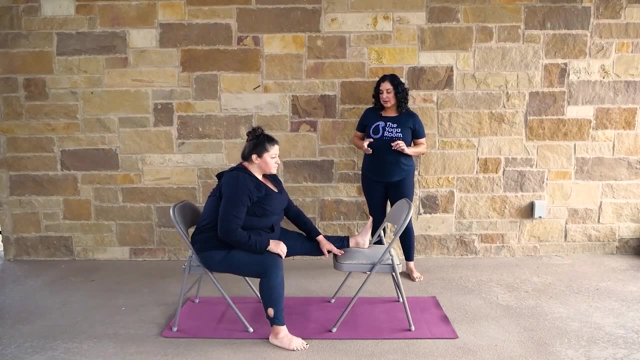 mat. so yeah, and then fold this direction rather than folding towards your leg, fold this way toward this side of the chair. is it different? yeah, yeah, you may feel sometimes, with this one, more stretching in the outer part of the leg, you may also feel it in a different. 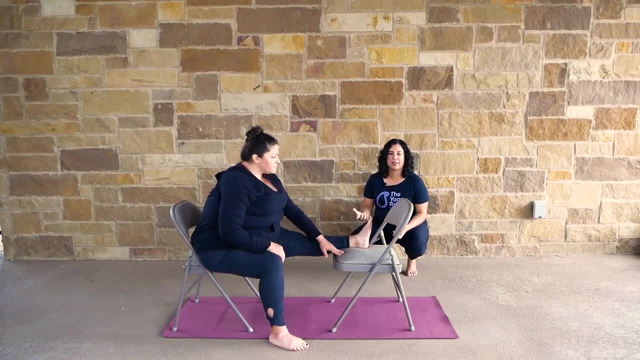 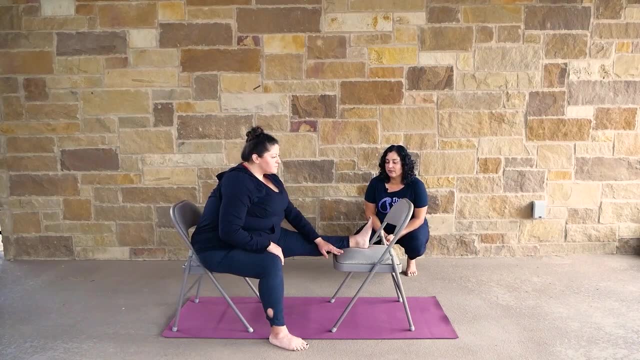 part. so maybe previously you were feeling more in the calf, now you're feeling more in the thigh, or something like that. every body is different, so you'll feel it in a different way. okay, when you're ready, go ahead and come on up and then set your left foot down. 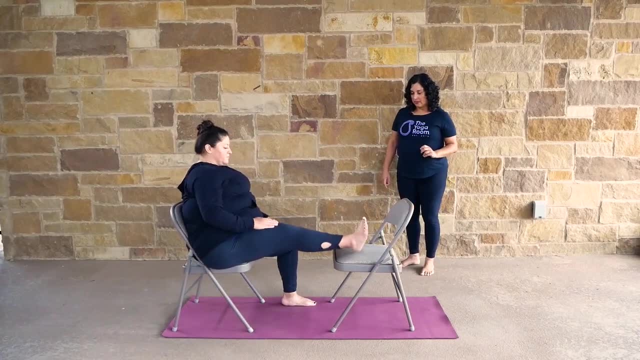 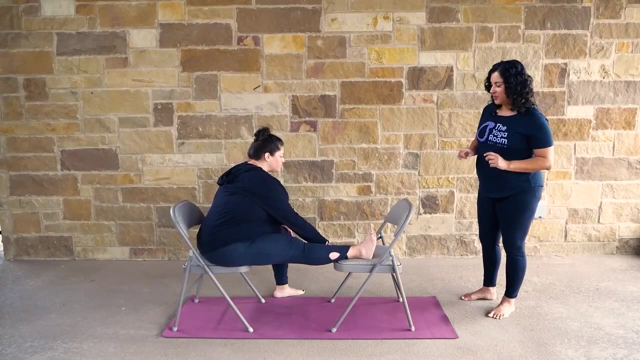 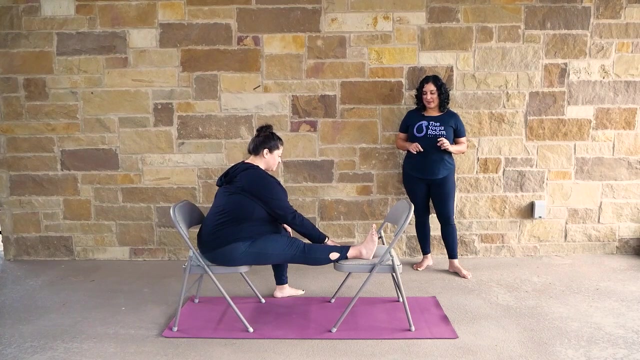 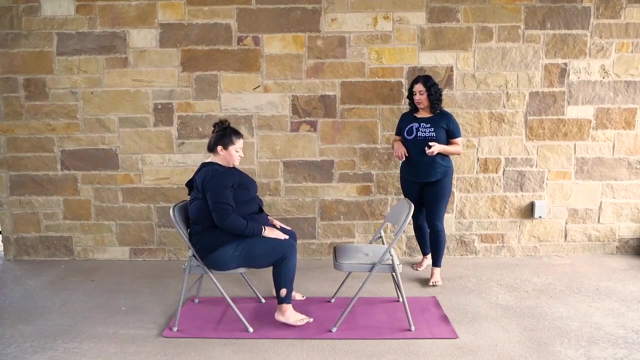 and we'll do the same thing with the right leg up. yeah, there you go, and then go ahead and fold this direction. this one looks tighter. all right, a few breaths here, maybe about three. okay, good, when you're ready, go ahead and come on up and you can set this foot down and then we're going to wrap up the practice. i'm 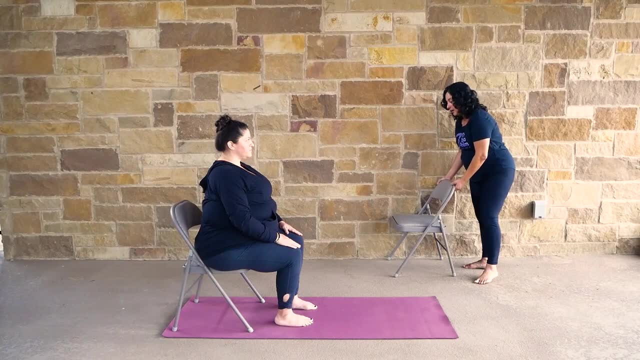 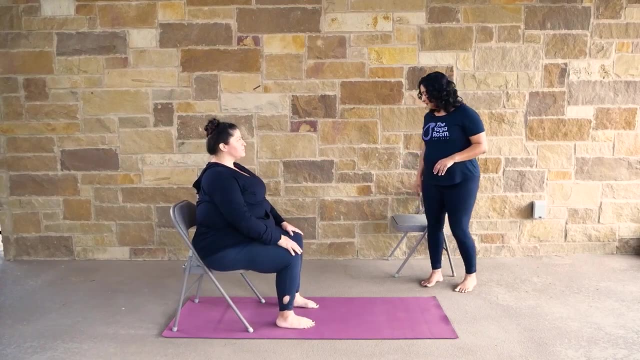 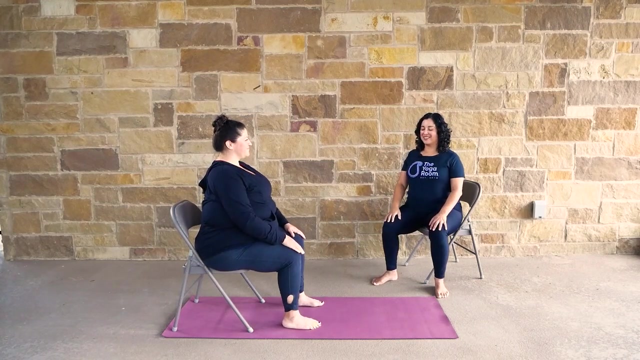 going to move this out of your way, um, with a little bit of. well, first let's actually do a couple of counter pose for that, so you can just shake your legs out a little bit, make sure they're comfortable, and then i'll sit here. we're going to, uh, do two last things. the last, the second to last one, is a little. 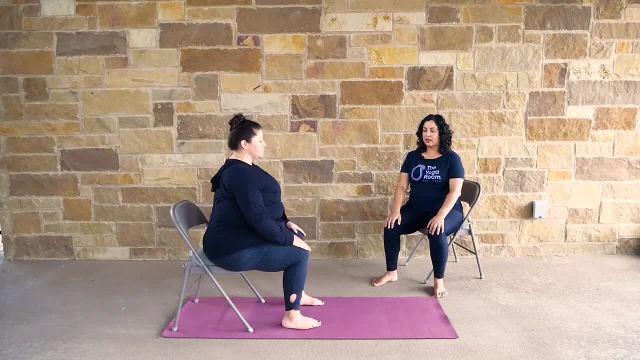 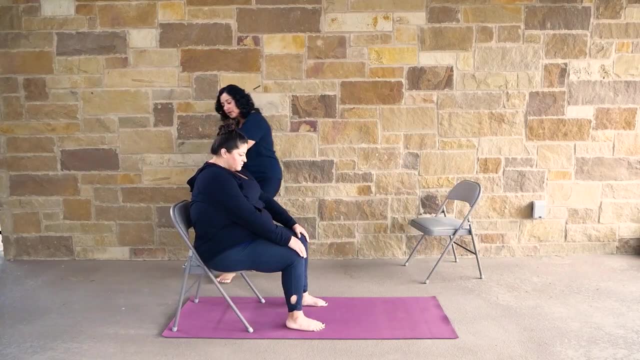 bit of work for your spine. so from this position here, hands on the knees, inhale, reach your chest up and then exhale and round your spine- perfect, and you're bringing your back toward the back of the chair, tucking your chin down a little bit. then next inhale, lift your chest up a. 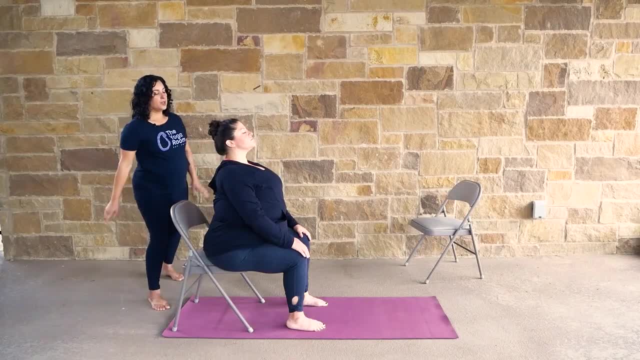 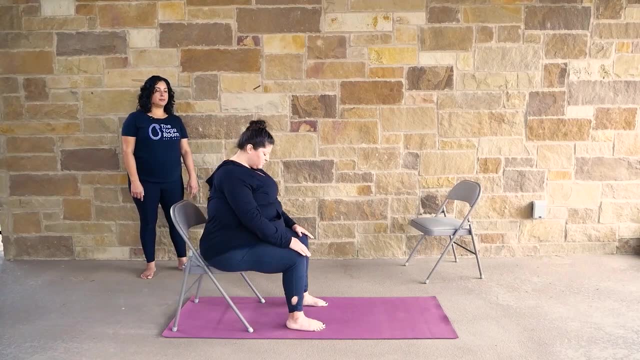 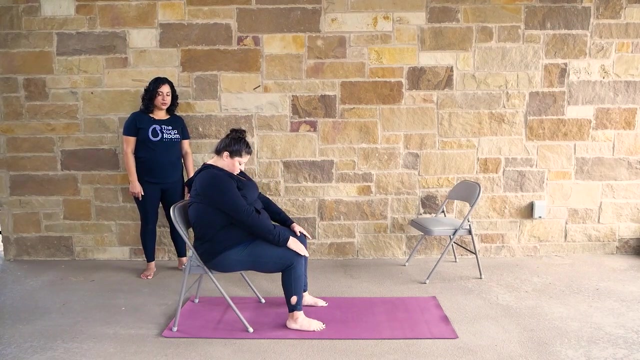 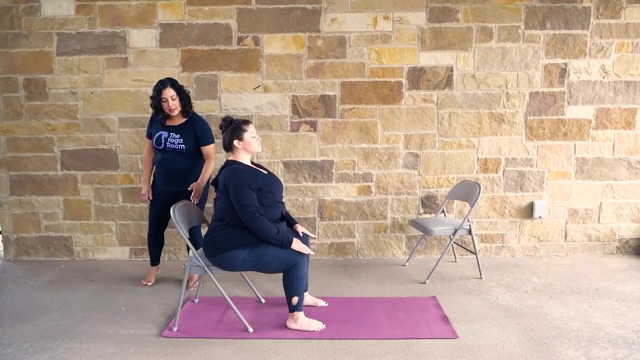 little back bend, keep relaxing your shoulders. down there you go. exhale, round your back, inhale and come up. chest lifts up, exhale and round. go ahead and do two more. go at your pace. you'll notice how denise is sat kind of up toward the front of the chair. that way she has space back. 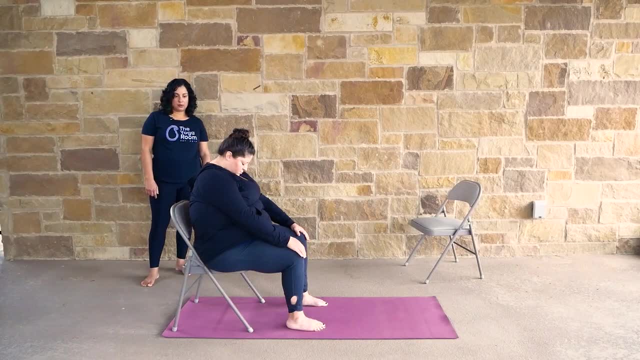 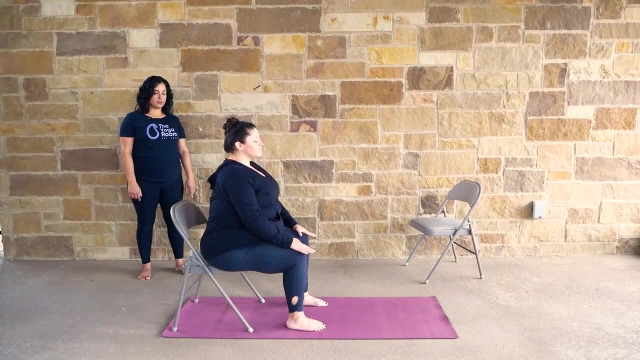 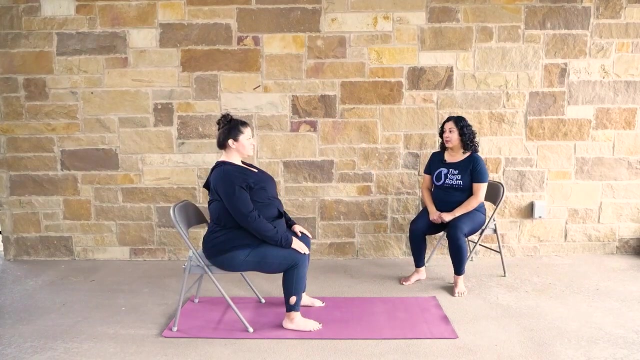 here when she's rounding her back. one more round, excellent- and then inhale back up to a neutral spine position. the last thing that we're going to work on is a little bit of movement for the neck, which is going to help reduce tension in your neck and in your shoulders, and also we're 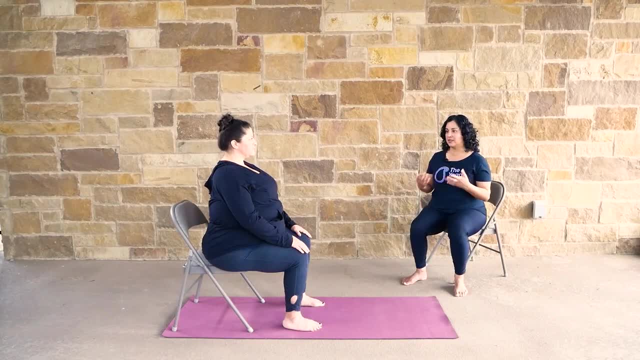 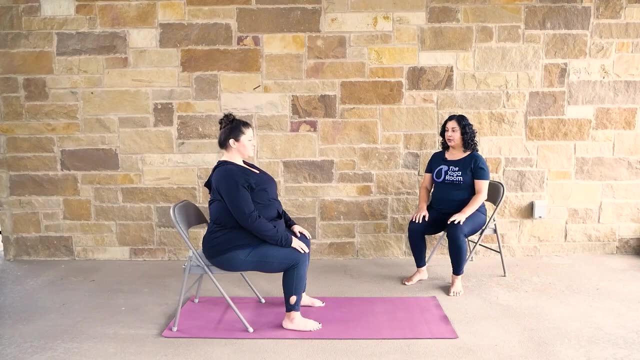 going to coordinate breathing with the movement so that we have the mindfulness benefits, and i'll get into the details of that in just a little bit. but you can go ahead and begin. so what you're going to do is, on an inhale, you're going to lift your 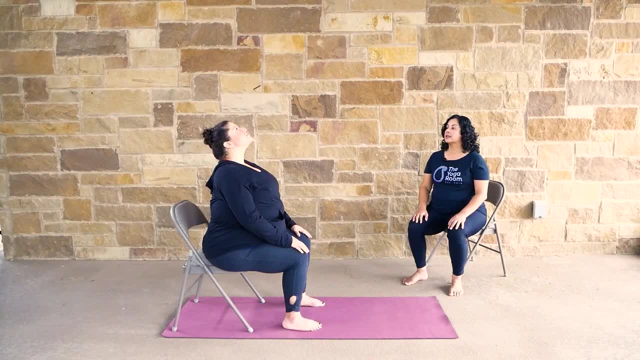 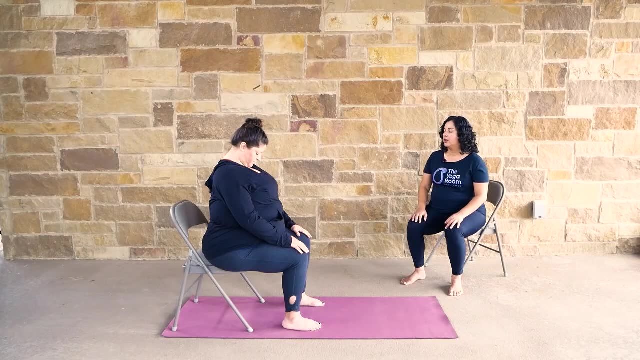 chin and you can face upward, and then, on an exhale, slowly lower your chin toward your chest and if you want to close your eyes here, that's perfectly fine. keep going at the pace of your breathing. inhaling up, exhaling down: both movements are smooth and as slow as is comfortable for you as you're doing this. the physical: 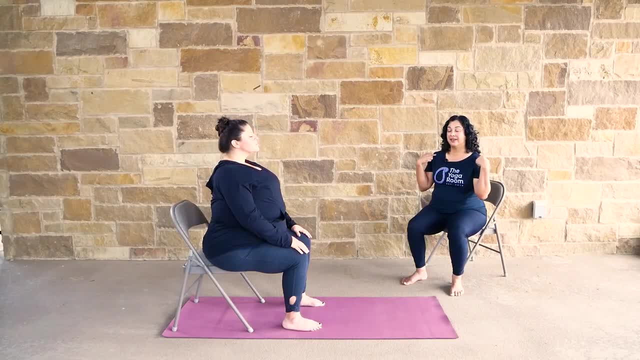 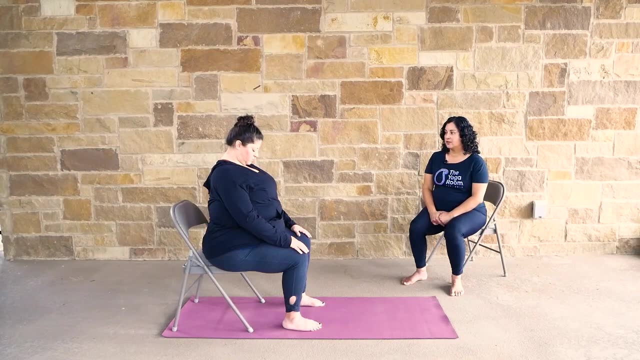 benefits are reduction of tension in your neck and in your shoulders and in your upper back, and then i was mentioning earlier about the mindfulness benefits. so as you're, you know, coordinating- there's lots of, lots of subtle things going on here. so you're coordinating the pace of your breath to the pace of your movement. 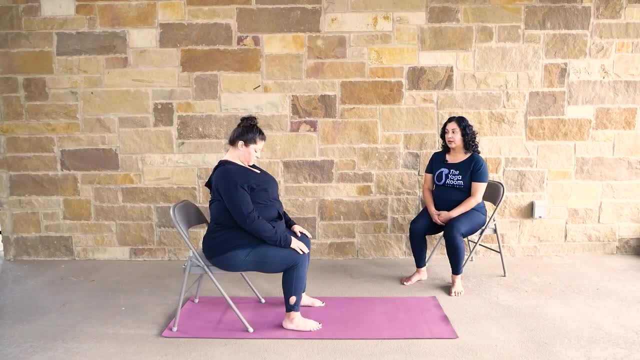 and you're keeping that in mind. you're present in order to keep all of that coordinated. and when we practice mindfulness in this kind of way, like we do generally in the yoga practice, we are calming the nervous system. and as we calm the nervous system, there are 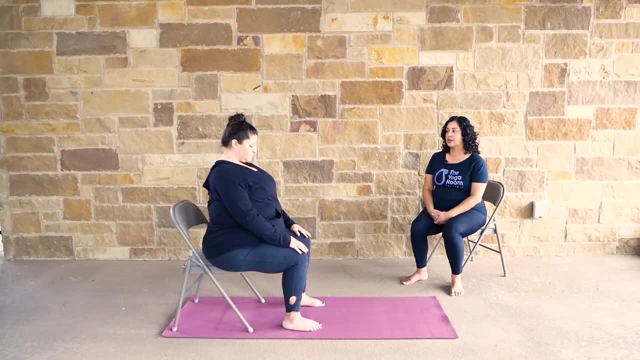 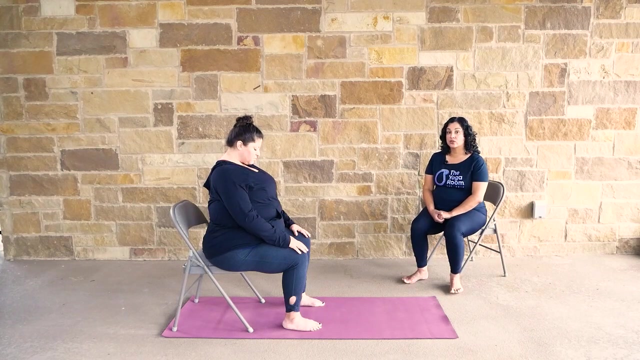 lots of benefits that happen. we have a reduction in stress hormones. we have, you know, just the general relaxation response in all of the systems of your body, and many diseases are known to be exacerbated by too much stress. and so if we're practicing mindfulness and calming our nervous systems, we're helping ourselves to be.